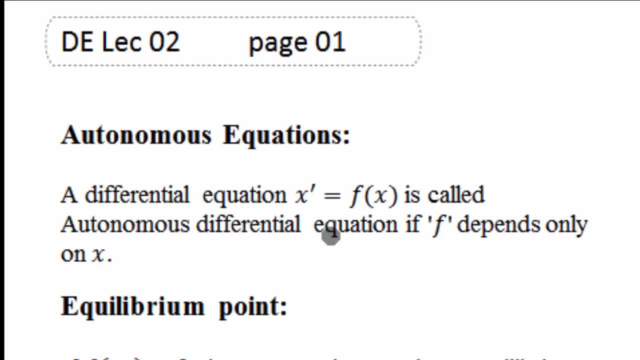 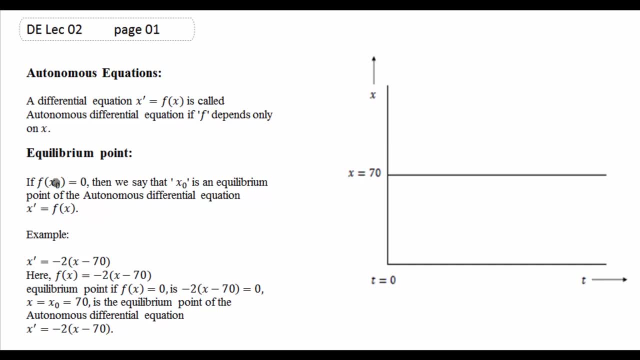 equation. So we will call such equation autonomous differential equation. We can take it like this-like: same renovation line that has å Same. And then after that there is an equilibrium point, one point on which situation, as we mentioned, all 4 functions in this equation are connected to another fixed number. Now 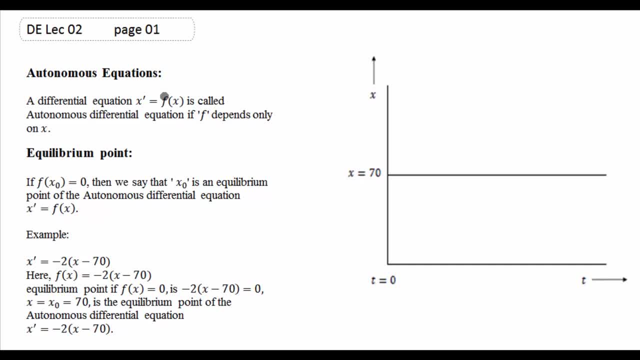 right side of the autonomous differential equation is 0,. that means whichever function lies in the right direction, If you form that function as equal to 0, then you will find the within that function's root. So whichever root, you can find the developers of that function. 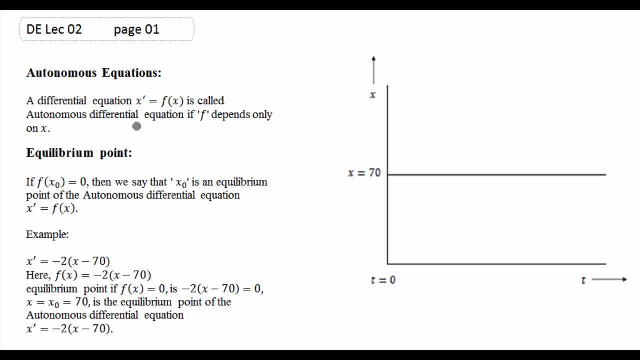 all the root there is is given autonomous differential equation of you defining one is the situation. n is not very convincing as well In this situation, remember that this function of frequencies equation will have an equilibrium point. As it is written, if f of x0 is equal to 0, then 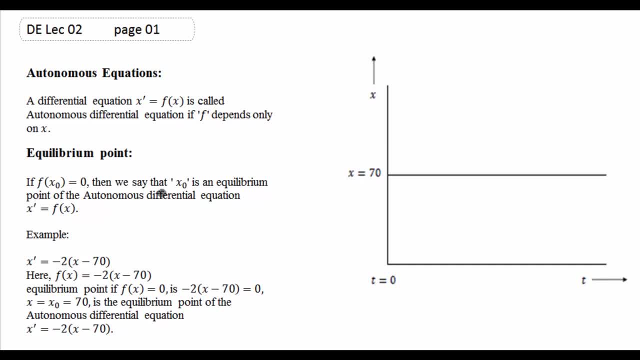 we say that x0 is an equilibrium point, Then we will say that the point at which the function value is 0 is an equilibrium point of the autonomous differential equation x prime equal to f of x. This is an example: x prime equal to minus 2 times x, minus 70.. Now look at the 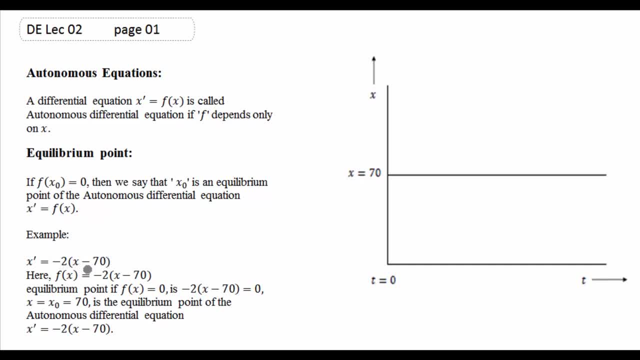 function on the right side. This is a function of x and x is a dependent variable. In this course we have taken x as a dependent variable and t as an independent variable. So this prime is, with respect to t, derivative. The function in this equation is minus 2 times x, minus 70.. When will the function be? 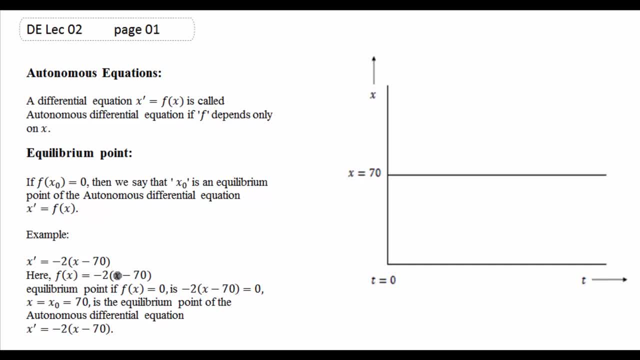 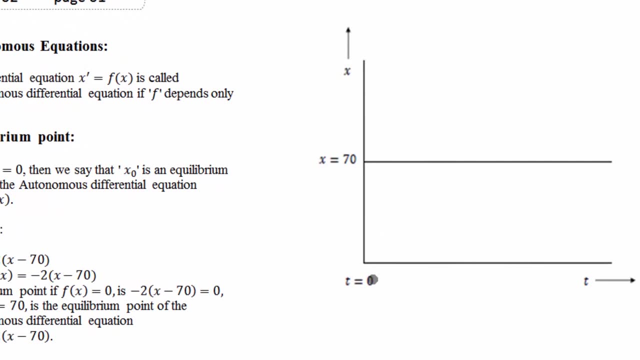 0, when you will take x as 70.. x equal to 70 is an equilibrium point for this differential equation. We have also graphically shown it here. This is the t-axis we have. So this is the equilibrium of the differential equation. 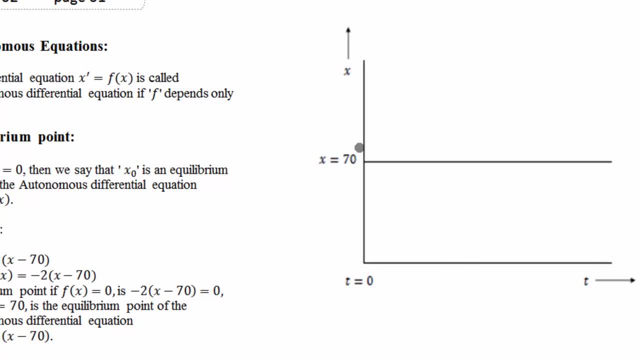 for independent variable and this is your dependent variable, which is x-axis, and on this we have taken that point. x equal to 70 and this line is free of t. there is no role of t whatever the value of t is. x is 70 and this is showing the equilibrium point. 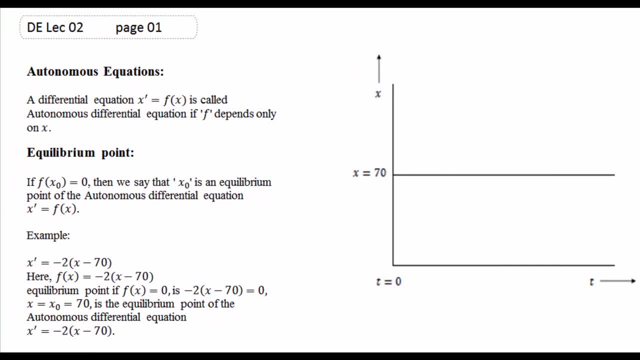 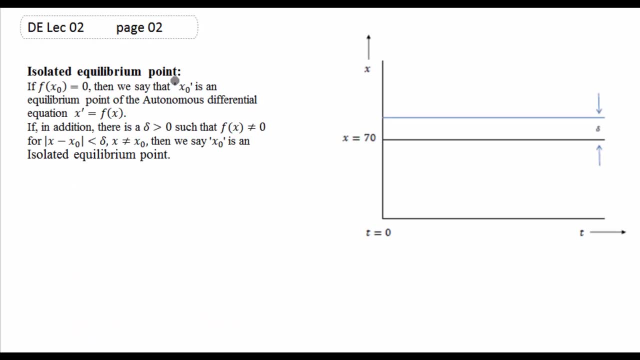 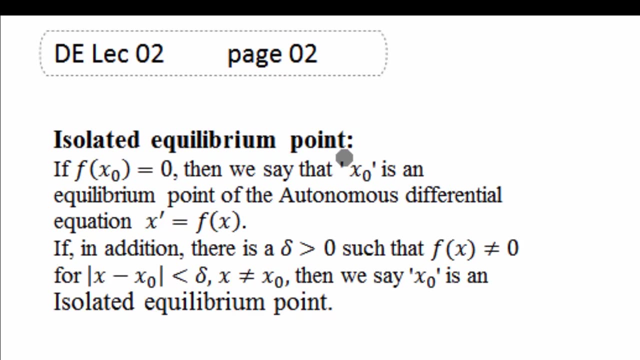 clear. next is isolated equilibrium point. isolated equilibrium point will be the point which will be in the neighborhood of equilibrium point, whether it is a small number from that point or a big number from that point. but when you will take the difference of those points with equilibrium point? 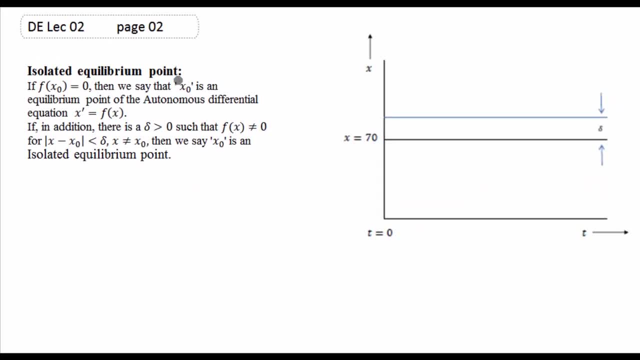 then that difference should be non-zero and positive and apart from that the value of function at those points should be non-zero. for example, we have checked at 70 that the value of function at 70 is zero. now I have taken some interval which I have denoted from delta. 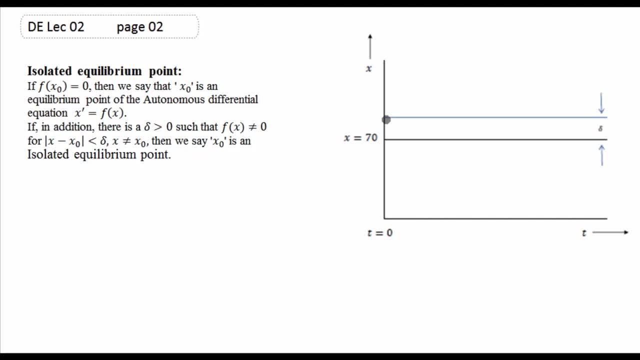 if this is 70, then you can call it 71, this whole area. what is its length? its length is 1 in this. I will take a point from here. for example, I can call it 70.9 when I will take the difference of 70.9 with 70. 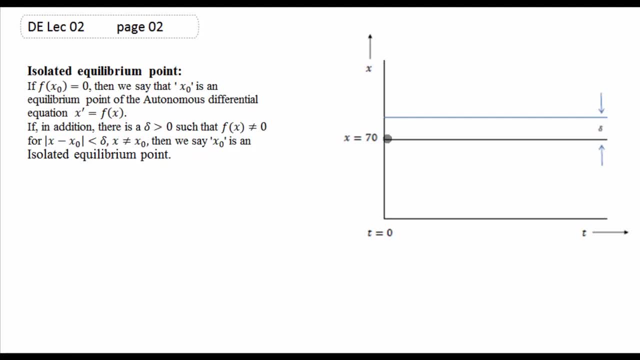 then what will I get? 0.9 and 0.9, because I have taken all this, that it is 1, so see that 0.9 is not zero, because the difference of these two, the point which you are taking from its neighborhood point, 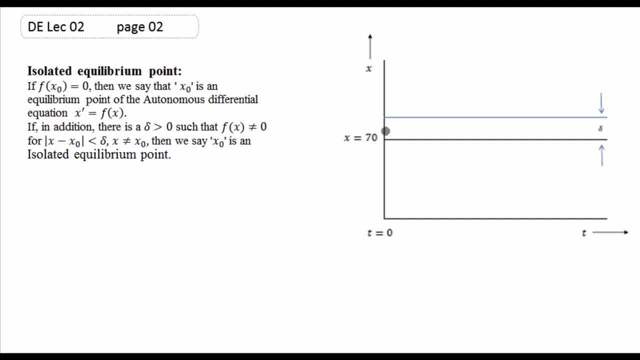 the difference of its over equilibrium point should not be zero. and then see this function, the function which we were given at the back. we have seen that this function was getting zero at 70. so when I will substitute 70.9 in it, then the value of the function will remain non-zero. 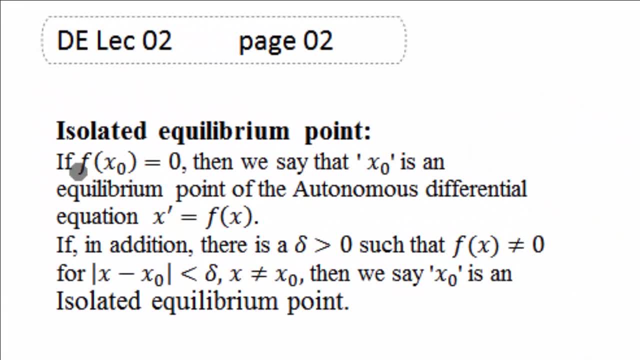 this is what is written in its definition. see this: if f of x0 is equal to zero, then we say that x0 is an equilibrium point at 70.9. we have already seen this in the autonomous differential equation, on which the value of the function is zero. 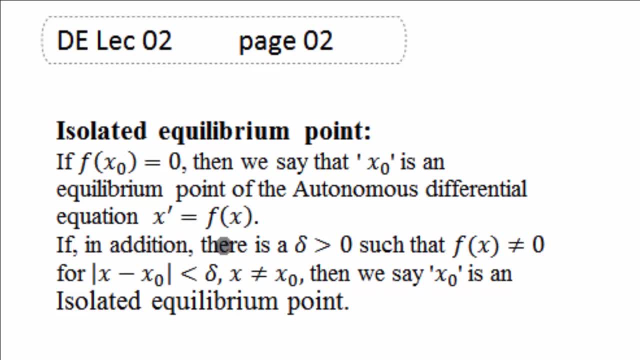 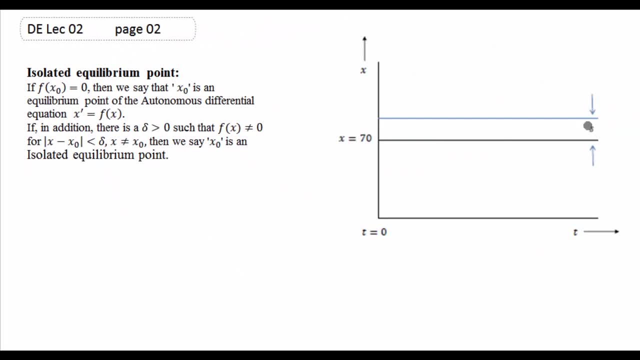 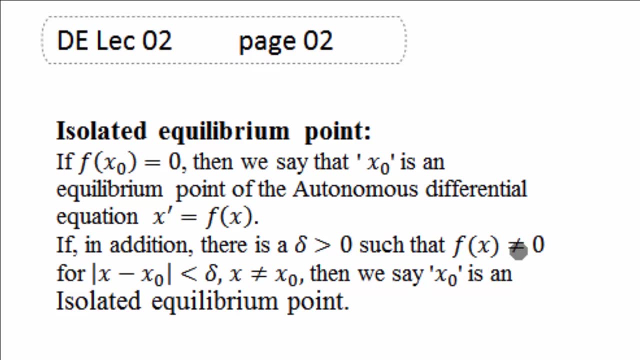 which we call the equilibrium point. if, in addition, there is a delta greater than zero, if you have a positive number, you have to take this from your choice, as I have taken this such that f of x not equal to zero, the function at some point should remain non-zero. 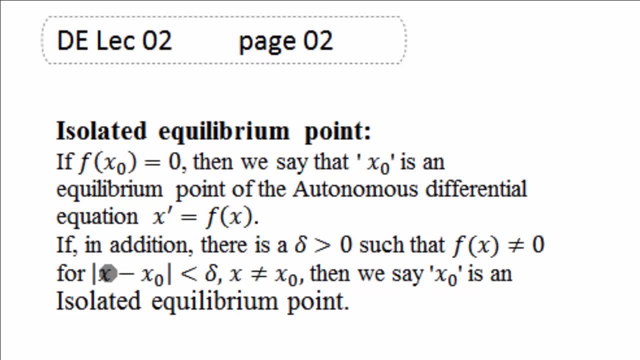 and what is that point? that point is that whose difference with the equilibrium point is below your taken delta. but because this model is being taken, so it will be positive because you have taken the positive delta, and then that point should also be different from the equilibrium point. 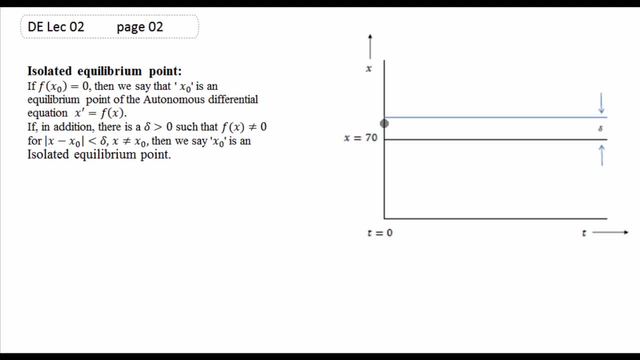 as we took here, 70.9, because it was different from 70, and on that the function will remain non-zero. so all those points whose difference with this will remain non-zero, and the function will also remain non-zero all those points of the equilibrium point. 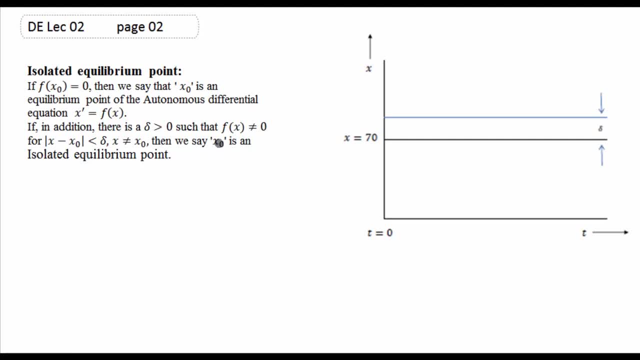 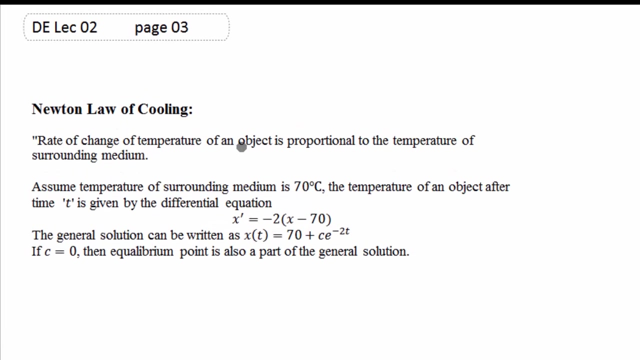 then we say that we can say that x0 is an isolated equilibrium point. we can also call x0 an isolated equilibrium point, and here in the neighborhood these points also exist. now let's see the next Newton law of cooling rate of change of temperature of an object. 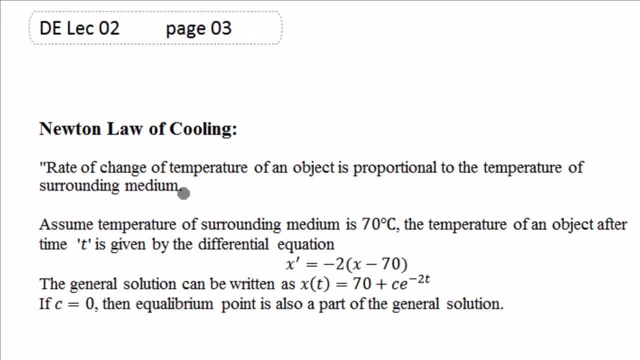 is proportional to the temperature of surrounding medium. Newton law of cooling says that if any object is lying in any medium, then, along with the object time As time passes, the temperature of the object becomes the same as that of the surrounding medium. If the temperature of the surrounding medium is high and the temperature of the object is low, 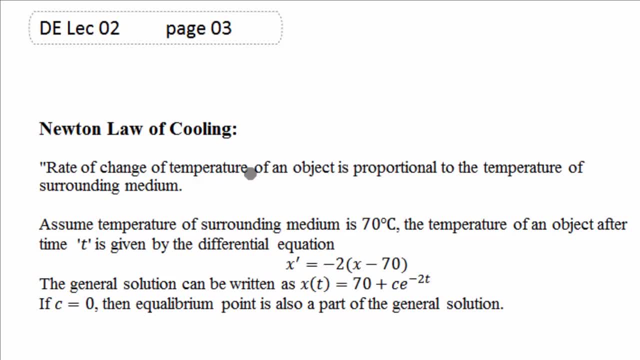 then the object will adopt the temperature of the surrounding medium along with the time, Its temperature will also be the same as that of the surrounding medium. If the temperature of the surrounding medium is low but the temperature of the object is high, then the temperature of the surrounding medium and the temperature of the object will be the same. 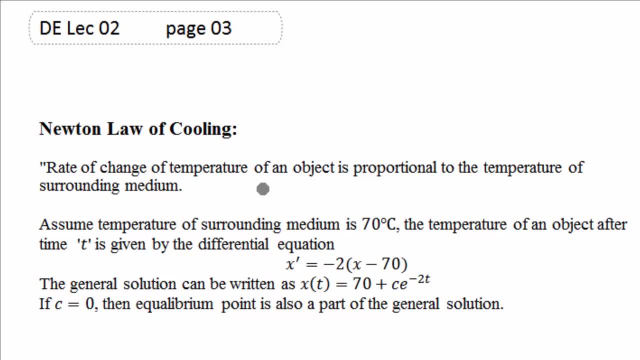 Newton's law of cooling says that in advanced countries the police also use Newton's law of cooling. For example, if a person is murdered in a closed room, the police come there late When they reach there, if they have to guess the time of the murder. 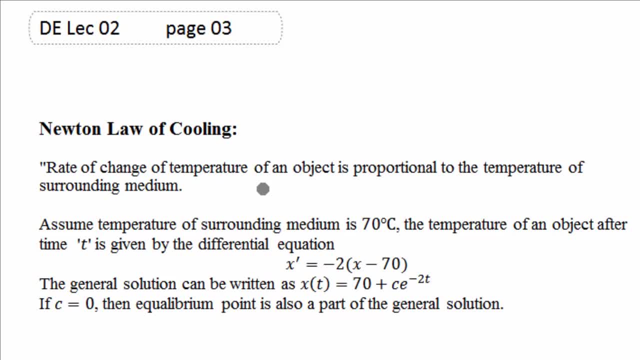 then they note these two things: They check the temperature of the dead body and the temperature of the surrounding medium. They use Newton's law of cooling to calculate the time of the murder. Assume the temperature of the surrounding medium. Assume that the temperature of the surrounding medium is 70 degrees centigrade. 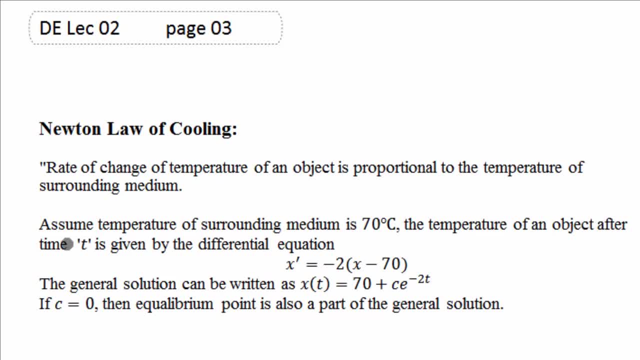 The temperature of an object after time t is given by The temperature of the object- is calculated by Newton's law of cooling. This is a linear first order differential equation In variable x. It has dependent variable x When you solve this by integrating factor. 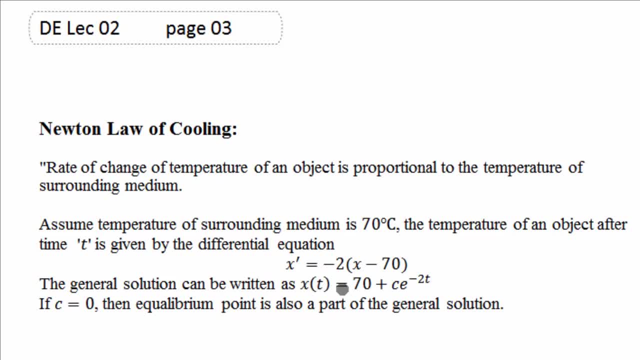 then you will get the general solution of this: x t equal to 70, plus c e raised to the power, minus 2 t. If you take this arbitrary constant as 0, then you will have x t equal to 70.. You know that 70 was the equilibrium point. 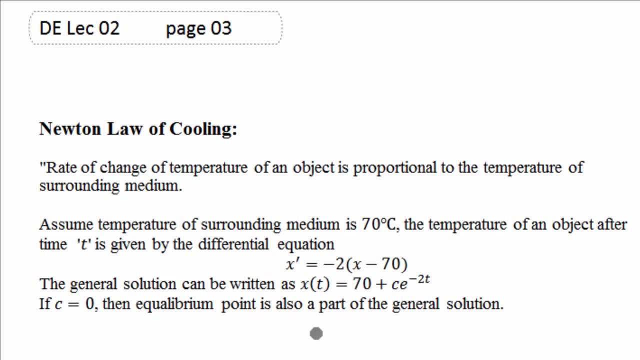 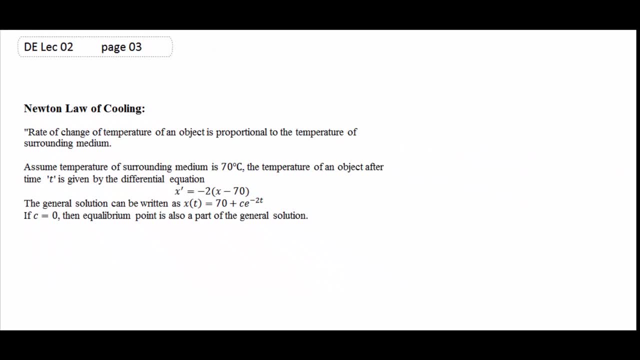 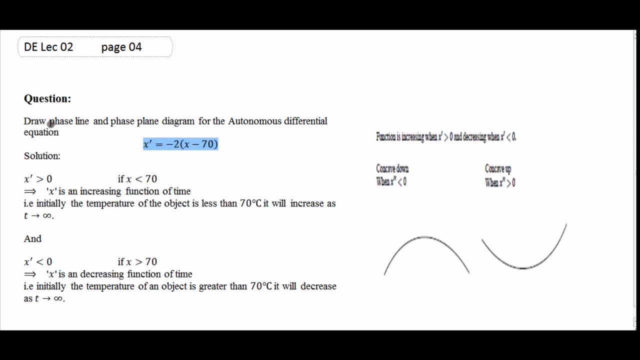 This means that the equilibrium point is also a part of the general solution. If c equal to 0,, then the equilibrium point is also a part of the general solution. Now we have counted a question here. What we have to do in this is: 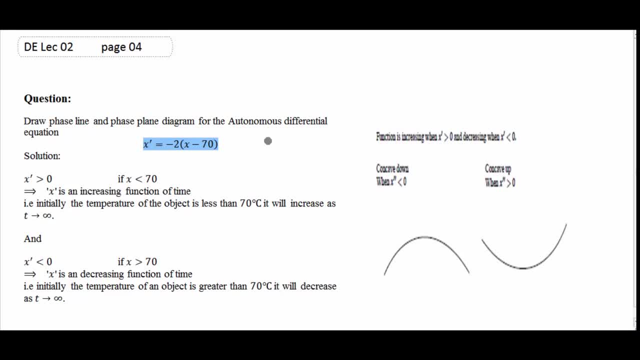 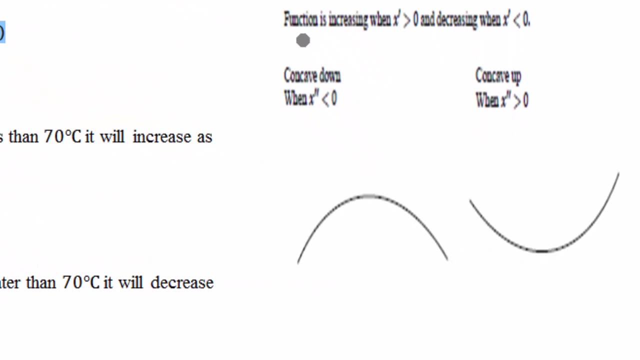 It is an autonomous differential equation. But what we have to do is For that we have to draw a phase plane diagram and a phase line diagram, And before that we have to see a concept. For example, there is a function If the first derivative of that function is: 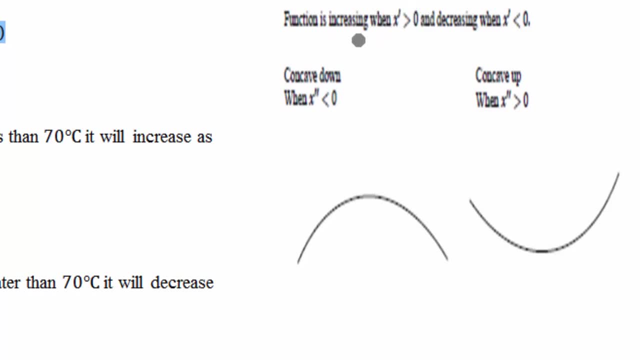 If it is positive, then that function is an increasing function. As the value of the independent variable increases, then the value of the dependent variable also increases. If the first derivative is negative- if it is less than 0, then it is a decreasing function. 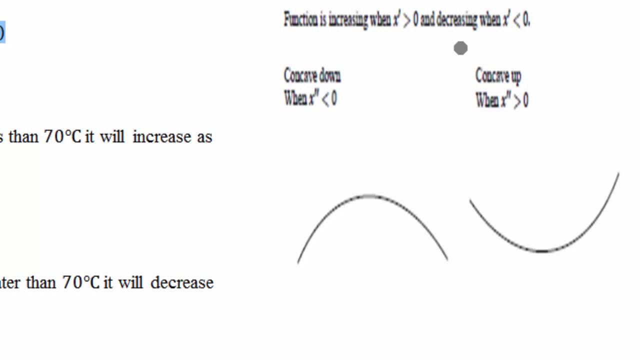 As the independent variable increases, then the dependent variable also decreases, Then the concavity. The concavity is related to the second derivative. If the second derivative of your function is negative, if it is less than 0,, then the figure that is formed is the concave down. 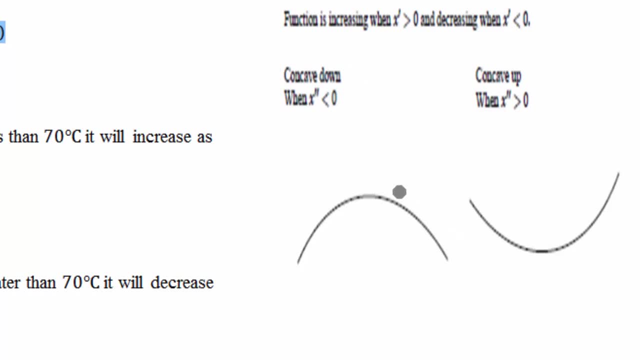 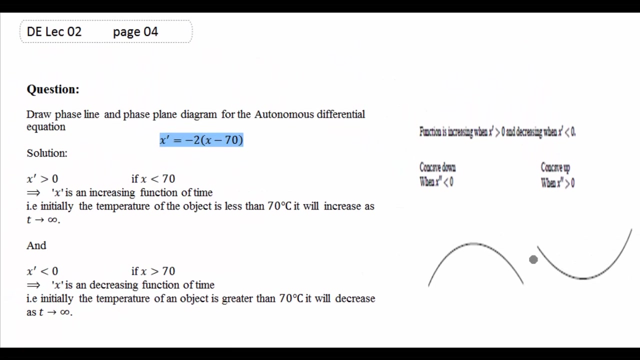 As shown here. This is the concave down. If the derivative of the function is, if the second derivative is positive, then we say that this is the concave up. This is the concave up. This concept should be clear to you. 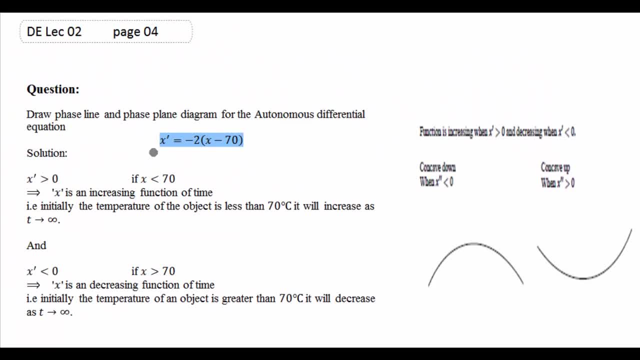 So here also in this problem, Newton's law of Coulomb, x prime equal to minus 2 into x minus 70. For this we have already found the equilibrium point. Its equilibrium point is 70.. Now first see its first derivative. 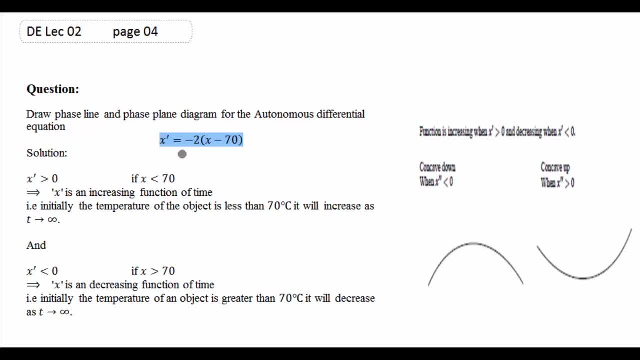 We have already known its first derivative, Because the solution of this you have to get is x. That is the first derivative of x. x will also be a function. For example, if you integrate it, then you will get x, So x will be equal to its integral. 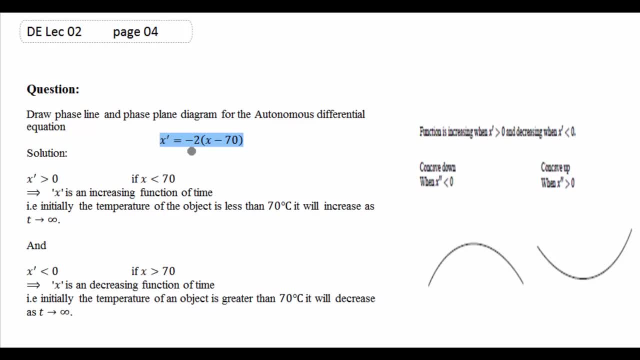 So it will be a function only. So its first derivative, see this, whose is equal to this Minus 2, into x minus 70.. Now 70 is the equilibrium point we have found. So according to 70, we check where the function is increasing. 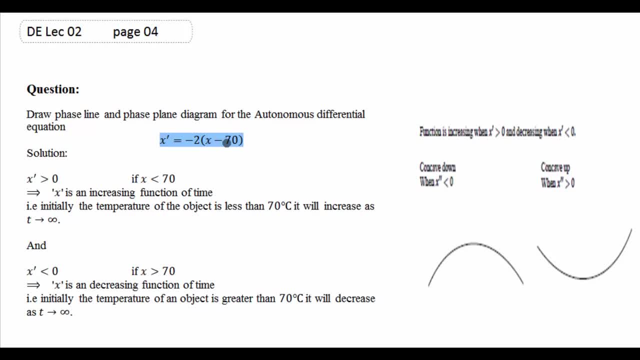 and where the function is decreasing. See here: if you substitute x less than 70,, in this x less than 70,, for example, you substitute 69. If you substitute 69,, then in the braces, in the parentheses. 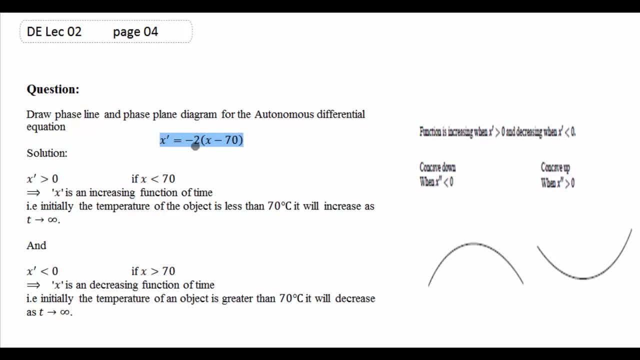 you will get negative 1.. That negative 1 and this negative 2, this will become positive 2. That is, whenever you take a number below 70, then you will get a positive number on the right side. This means that what will be your x prime? 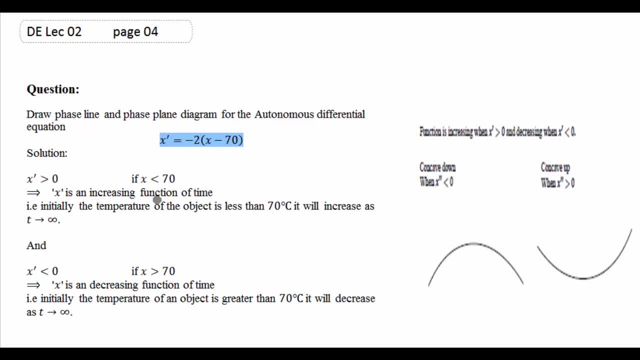 Positive greater than 0. So when it is greater than 0, then x is an increasing function of what Of time. Initially, the temperature of the object is less than 70 degrees. It will increase as t approaches to infinity. 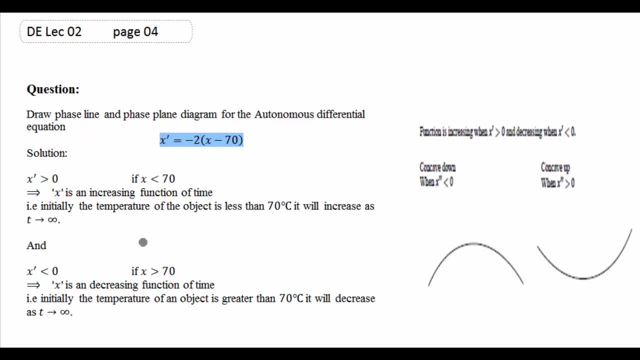 Because we are saying Newton's graph pool. So according to that, it is being said that if the temperature of the object is below 70, whereas the temperature of the surrounding medium was 70,, then what will happen As time passes, then the temperature of the object? 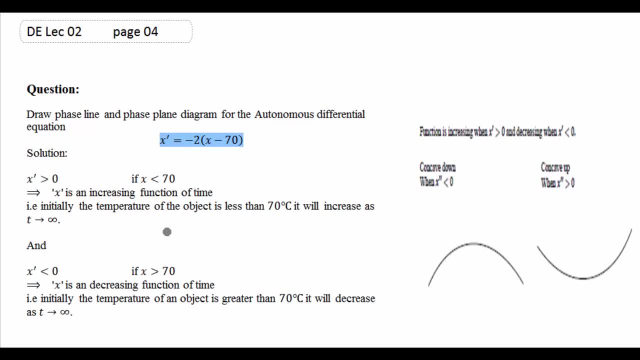 will also be equal to the temperature of the surrounding medium. In the same way, if we substitute x greater than 70 in this, if we substitute x greater than 70,, for example, if we substitute 71,, then in the parenthesis: 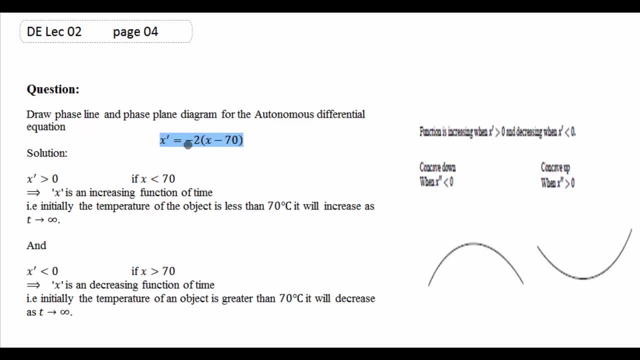 you will get positive 1.. Positive 1 will be minus 2 times minus 2.. This means that whenever you substitute a number greater than 70 in this, then you will get a negative on the right side. If you get a negative, 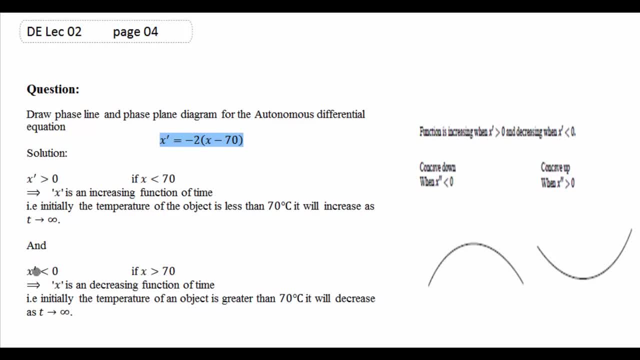 then your x prime first derivative will be less than 0. This will decrease your function. x is a decreasing function of time. Initially, the temperature of an object is greater than 70 degrees. The temperature of the object was greater than 70 degrees. 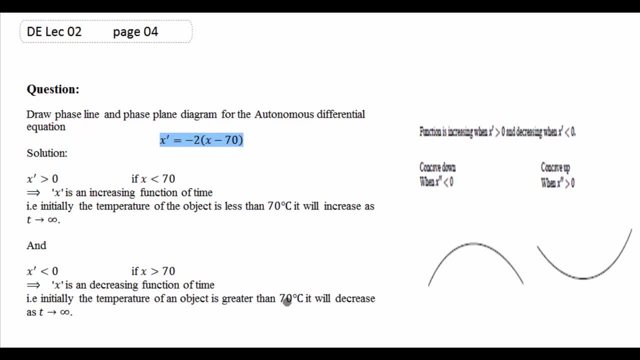 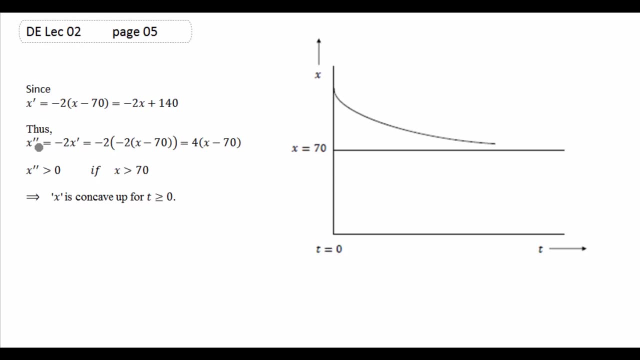 Because when we have seen this, we have taken 71 at that time also. Then what will happen? It will decrease, It will come close to 70.. Okay, Now look at this. After this, what did we do? We found its second derivative. 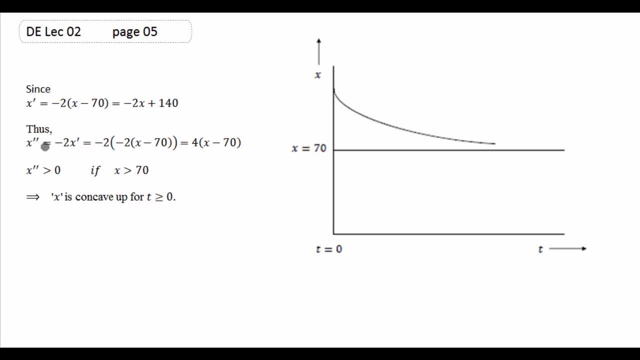 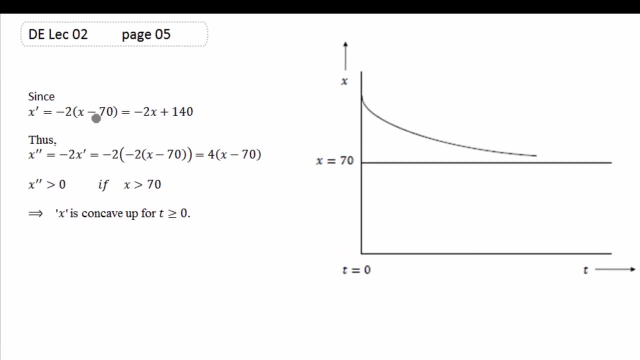 So that we can check its concavity at these two intervals: less than 70 and greater than 70.. So this was your x prime equal to minus 2 into x minus 70. So we multiplied it by minus 2.. So minus 2x plus 140. 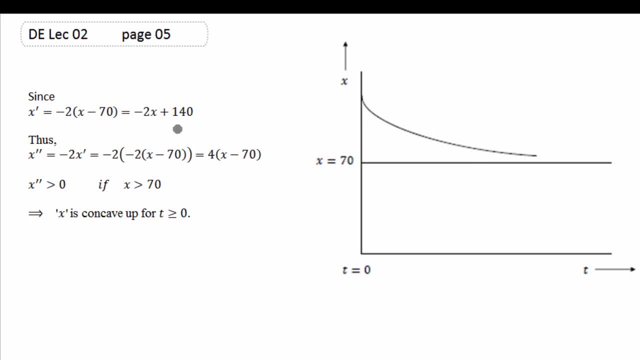 I took its second derivative with respect to time, With respect to time, So this became x double prime, equal to what will be the derivative here, Minus 2x prime, And minus 2 is the value of x prime. again, We will put it in this: 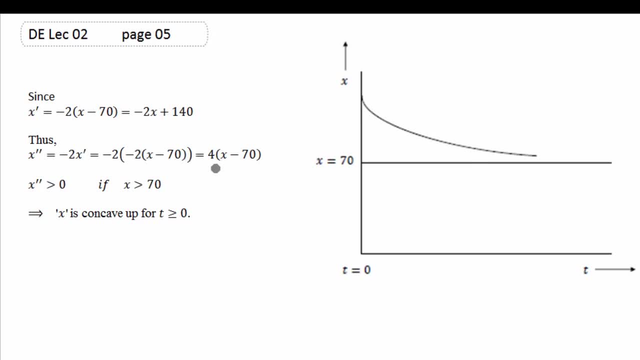 So when you simplify this, you will get 4 into x minus 70. Now again, you have to take the same interval: Greater than 70 or less than 70. Now see if you take x greater than 70. In this, x greater than 70.. 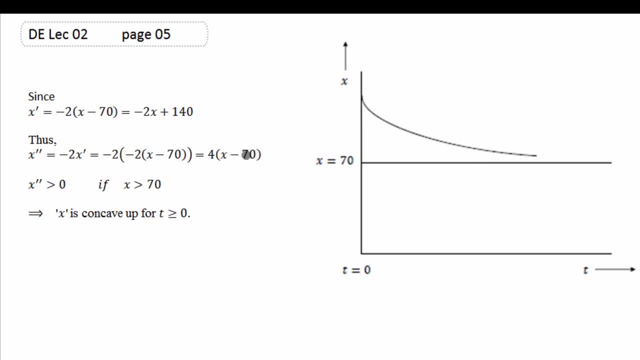 For example, if we keep 70 as 1, then you will get 1 in the parenthesis, 1, 4 times positive, 4.. So your second derivative is positive. Second derivative positive means that it will be concave up. The graph will be concave up. 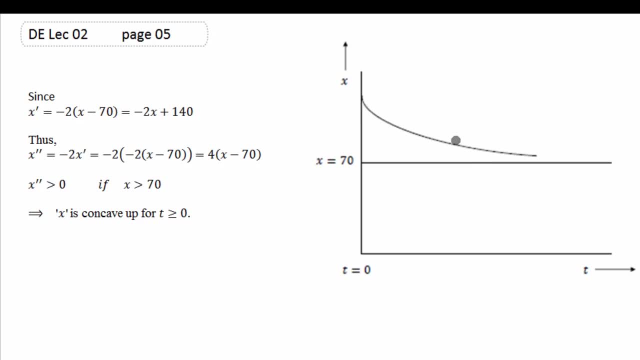 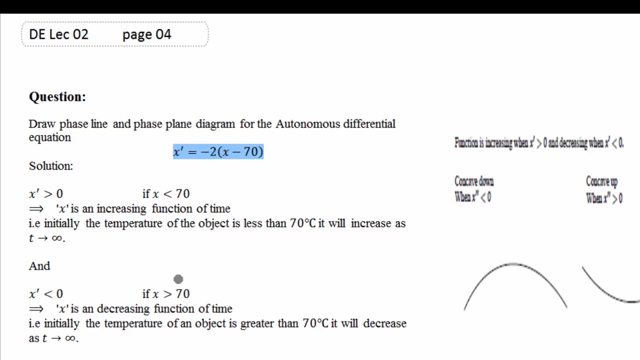 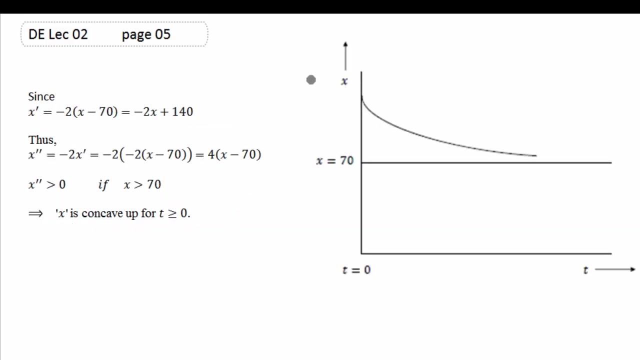 So see this- We have already checked this in the last slide- When x is greater than 70,. greater than 70, then the function decreases, But when x is greater than 70, then it is concave up. This figure is showing you that it is concave up. 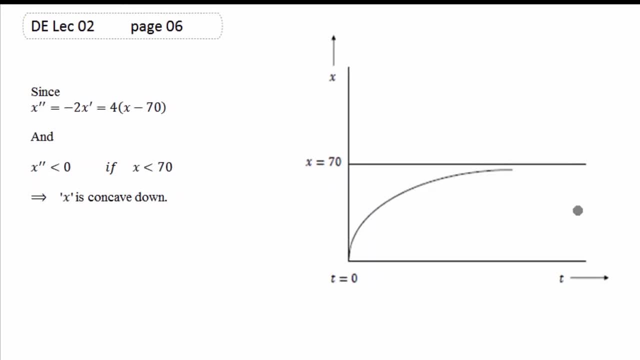 Now we will see the second interval This: If x is less than 70, in this you substitute less than 70, 69,, then you will get a negative number, Negative 1. Negative 1, 4 times negative 4.. 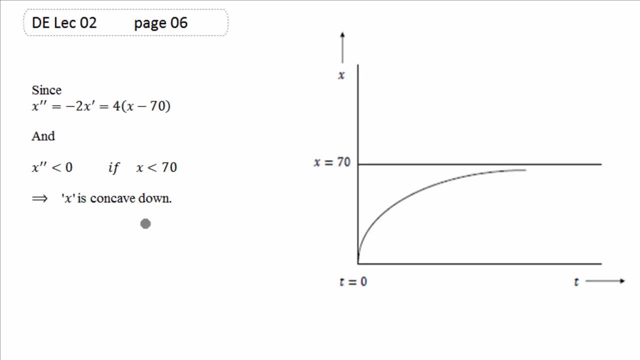 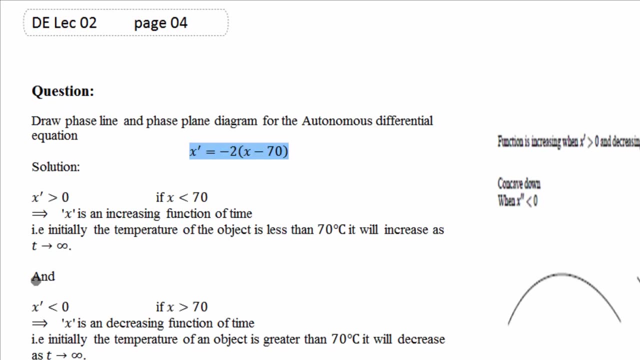 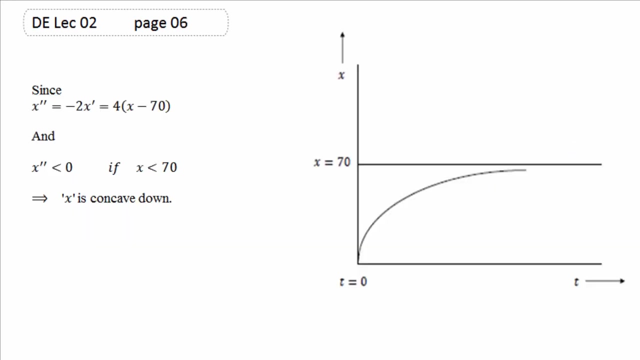 So x double prime will be less than 0. This means that it is concave down, Concave down, Whereas in this interval the function was increasing. The function was increasing at x less than 70. But what is remaining? Concave down. 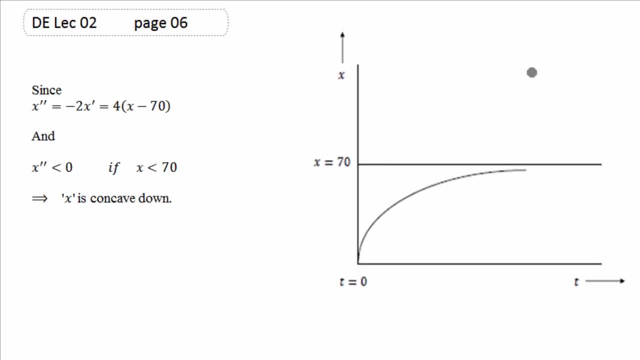 For that this figure will be made. Okay, The function is increasing. As you see here, t is 0.. As you go ahead, t is increasing And as you are going see, your graph is also increasing. This is the value of x. 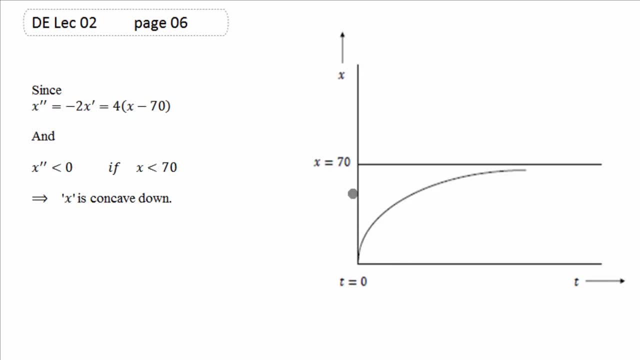 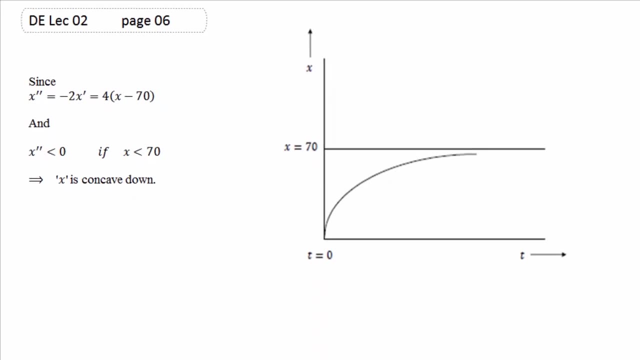 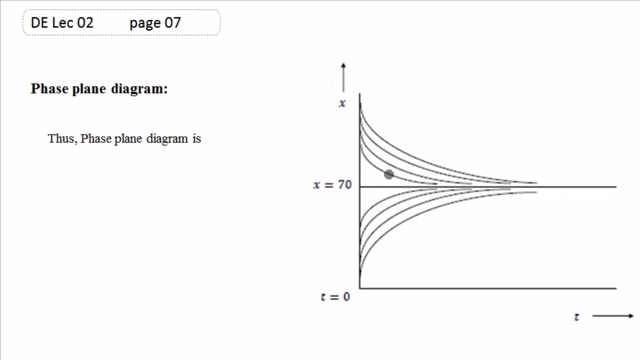 So, as you are going here, this is also going up. Okay, So this is increasing, but it is concave down, Clear so far, Okay. After this, we will be able to make phase plane diagram. We have taken different solutions for this. 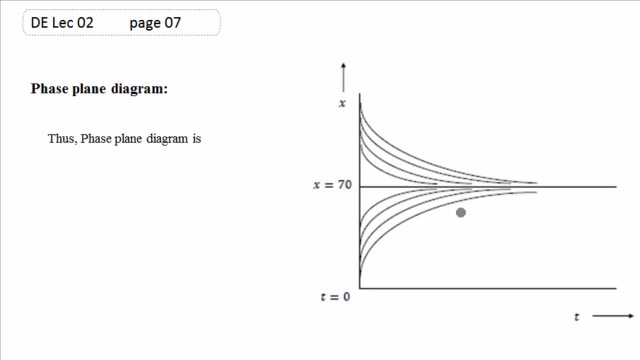 Similarly concave up and concave down, which we have seen one by one at the back. So this will become for this problem, for Newton law of cooling phase plane diagram. I hope that you have understood this, Because at the back 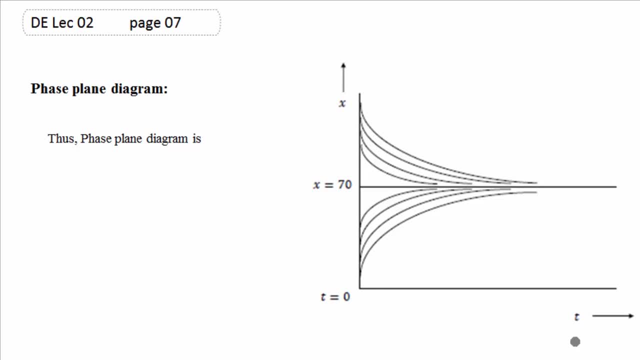 briefly these two steps. we have done a big graphical check And after that what you have to do is you have to increase the graph. First, we have seen one by one graph. Now we have done four by four graphs. 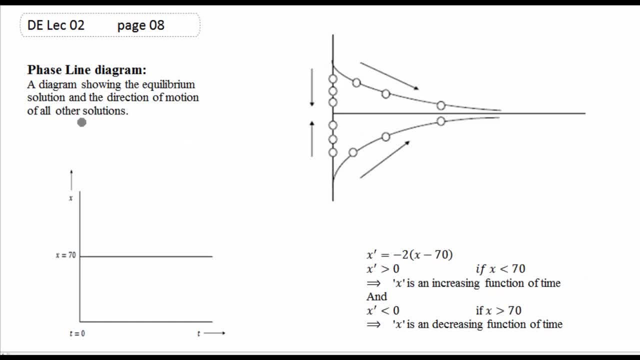 Now the second thing. we have seen the phase plane diagram, Now the phase line diagram. What is the phase line diagram? A diagram showing the equilibrium solution and the direction of motion of all other solutions. So a diagram showing the equilibrium solution. 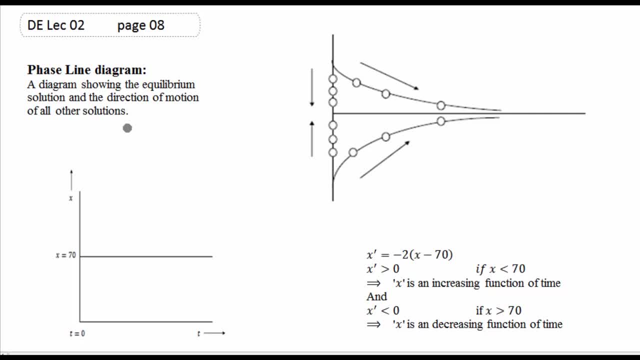 and the direction of motion of all other solutions that exist besides it. Look at this: This was your, this was your equilibrium point. So we have seen this. We have drawn these two solutions. Now pay attention to its trajectory, When this is the trajectory. 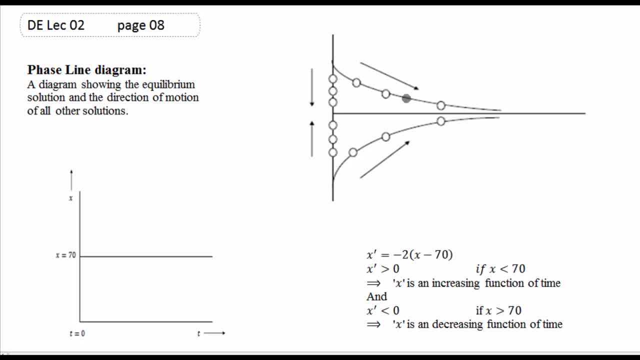 because this is the function. it is up, but the function is decreasing At this interval when your x is greater than 70, we have seen this in the back. Otherwise you can go from there again and see. So see, this is the decreasing function. 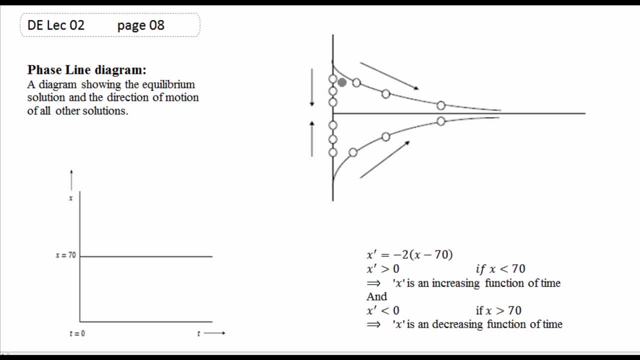 So when, if you see here, its shadow is this, This is its shadow. When you reach here, its shadow is this. Similarly, when you reach here, its shadow is this: If you talk about this, then in this: 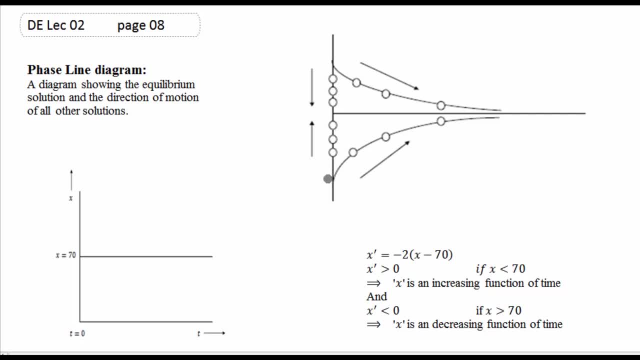 what is this interval? x is less than 70.. So in x less than 70, your graph is: it is concave down, but the function is increasing function. So see, when we reach here, its trajectory is this: 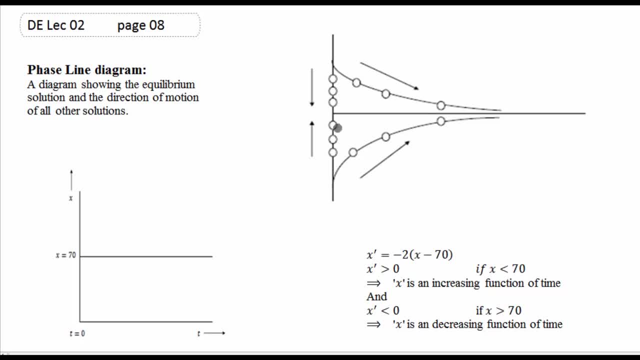 its trajectory is this and its trajectory is this. This arrow is showing that this is decreasing and this one is increasing. Otherwise, see from here. we have written all this, We have discussed this in the back, That at this interval, when x is less than 70,. 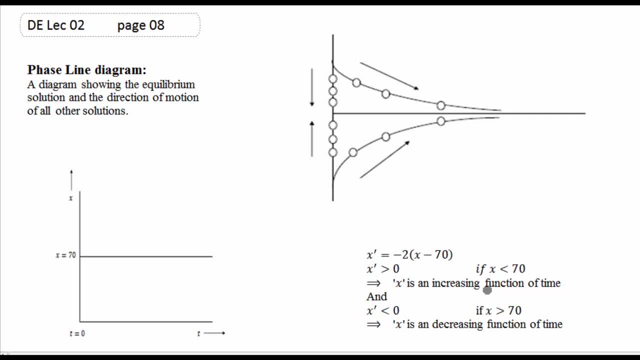 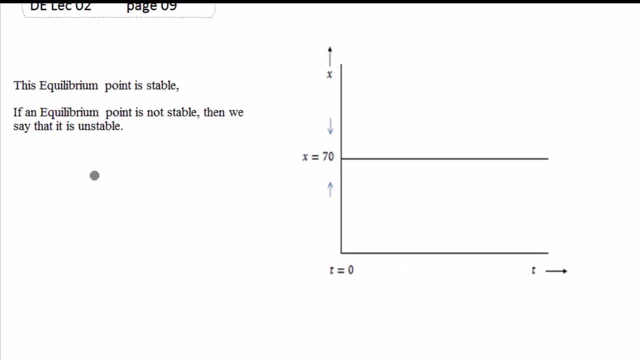 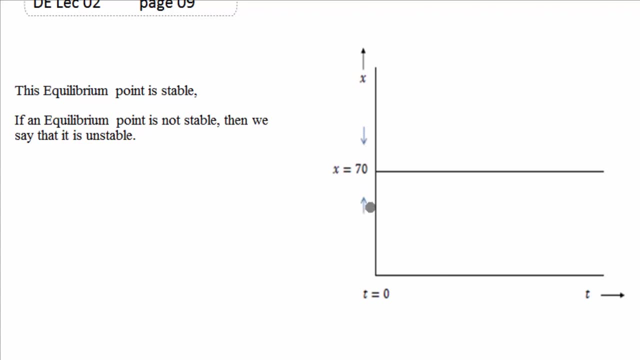 then what is this? It is increasing When x is greater than 70, then what is this? It is decreasing. Now, in the last figure we saw that one arrow is coming down and the other is going up. So when, at some equilibrium point, 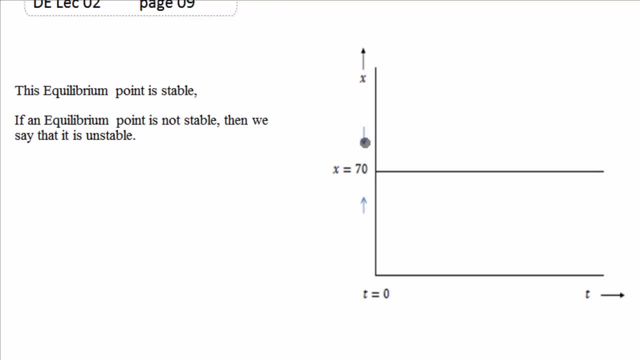 this situation is being created: that on one side the function is increasing and on the other side it is decreasing. On one side it is concave up and on the other side it is concave down. So then, 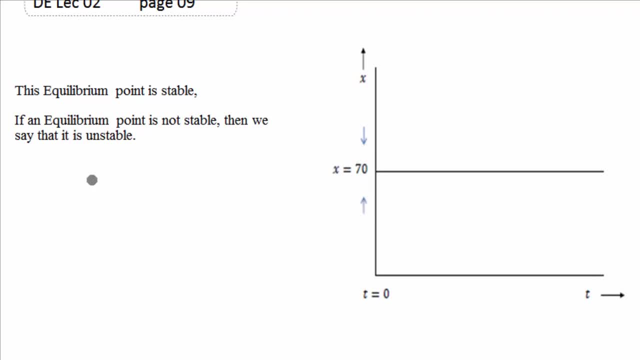 that equilibrium point, we say that this equilibrium point is a stable equilibrium point. This equilibrium point is stable. If an equilibrium point is not stable, then we say that it is unstable. If there was only one point in this, then that is your stable point. 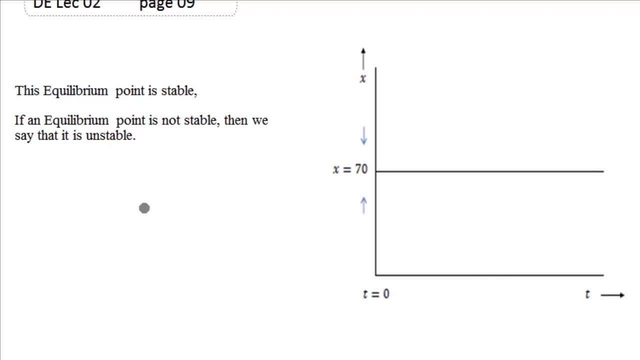 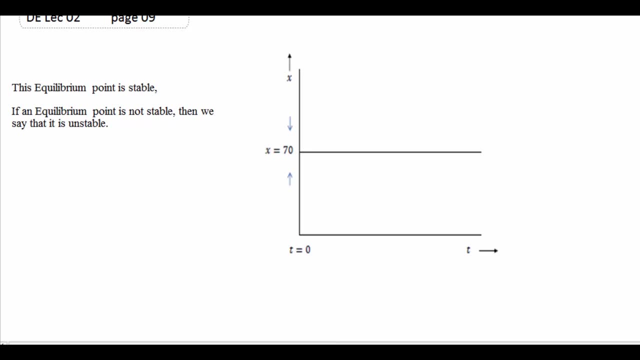 If there were more points, then maybe one or two of them are stable. At least one or two of them are unstable, So I can show you that too. After this, what did we do? The behavior of the same phase line diagram. 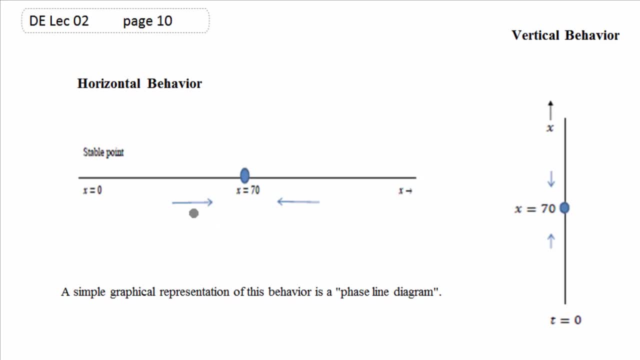 was also seen horizontally and vertically. See this: This is a stable point. This, This is just a figure. There is no description on this. We have already done all the description. at the back, A simple graphical representation of this behavior is a phase line diagram. 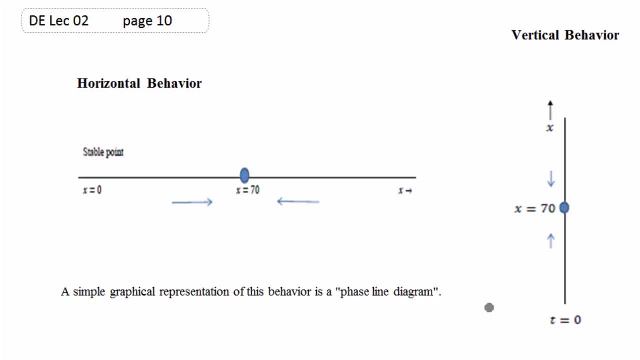 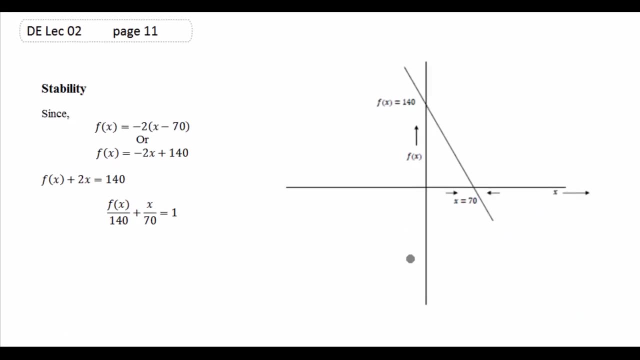 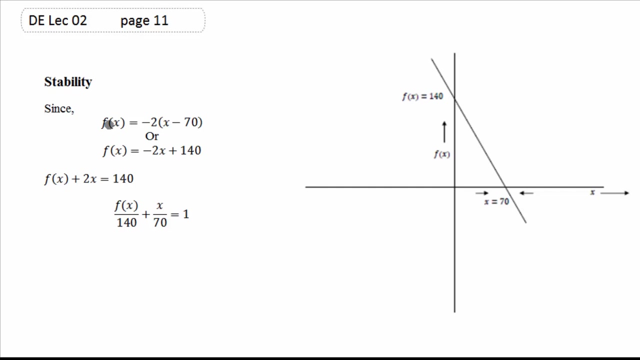 Whatever the graphical representation of that behavior is, that is what we call phase line diagram. Now look here. Here also we have seen stability. This was the function on the right-hand side. The given autonomous differential equation of f of x equals minus 2. 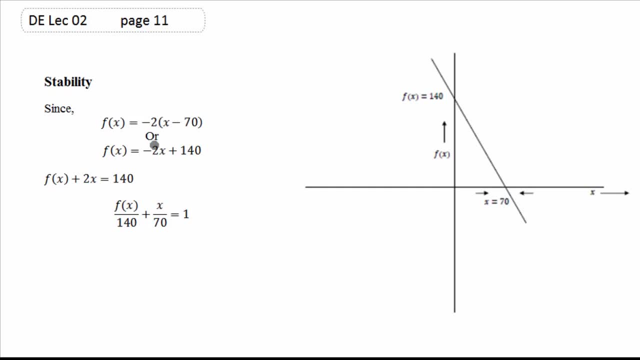 into x minus 70. I multiplied this So I got this. Now I took this variable and brought it to this side. I divided it at 140.. So I got this equation. This equation is in lower classes. If you get this type of equation. 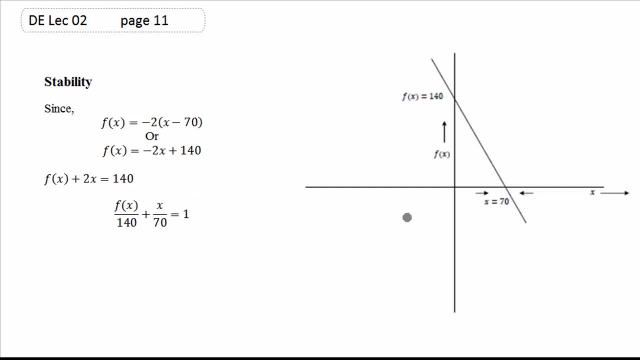 then you can represent it graphically very quickly. Now look, If I take f of x as 0.. f of x is on your vertical axis, x is on your horizontal axis. If I take this as 0, then I will get a point. 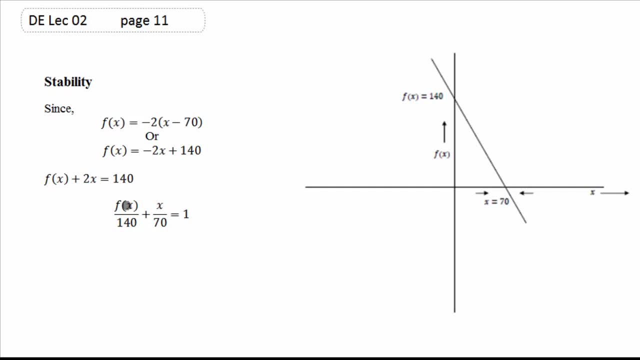 on the horizontal axis. If this is 0 on the horizontal axis, it means that all the first terms will be 0.. What will remain? x by 70, equal to 1.. So I will get x as 70.. I got x as 70.. 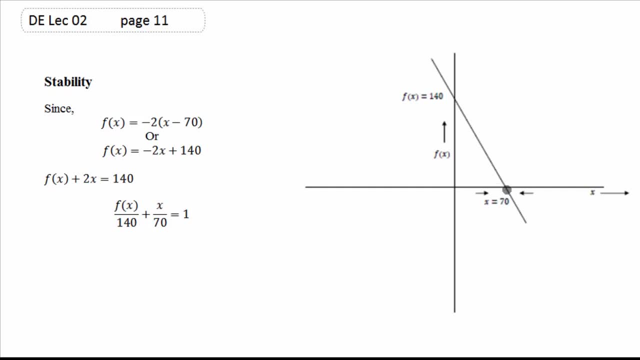 Because on this horizontal axis f of x is 0 and x is 70.. Similarly, if I take this as 0, then all the terms will be 0.. f of x by 140 equal to 1.. So I got f of x as 140. 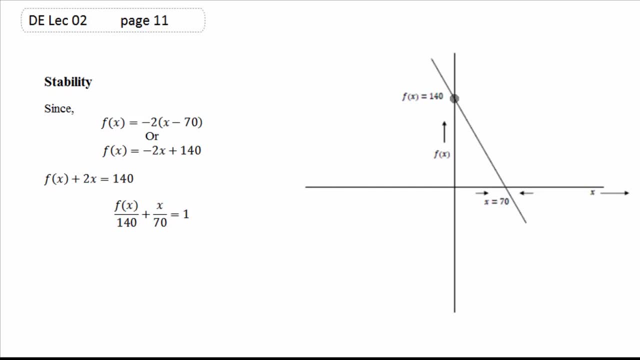 This is what I got. If you find two points, one on the vertical axis and one on the horizontal axis, then you can represent them graphically. So we have represented them graphically. Now look, All this is less than 70.. 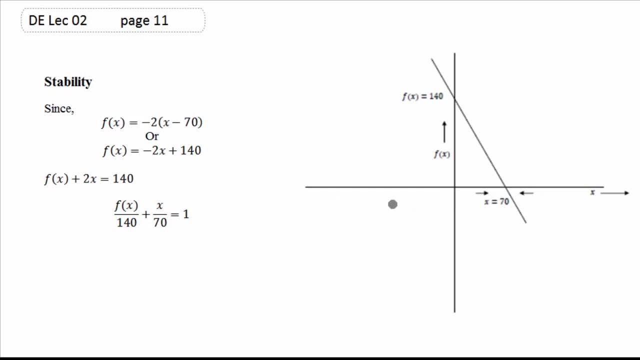 All this, x is less than 70.. So, whenever your x is less than 70, then look at this graph. This is above the horizontal axis. That means what is positive in the values of f of x. Similarly, at this interval. 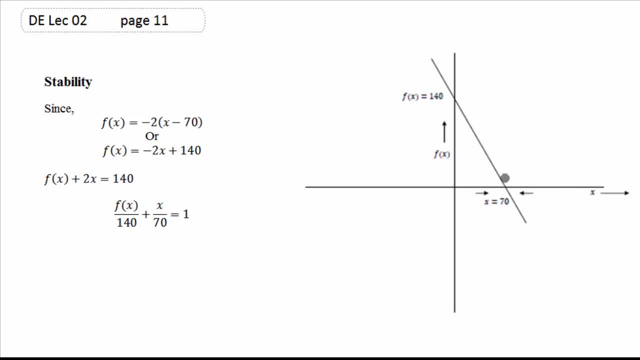 where x is greater than 70,, then what happens to your f of x Below the horizontal axis? So what did we find out from this? Whenever your function is less than 70, the function will be above the horizontal axis. So how will you draw it? 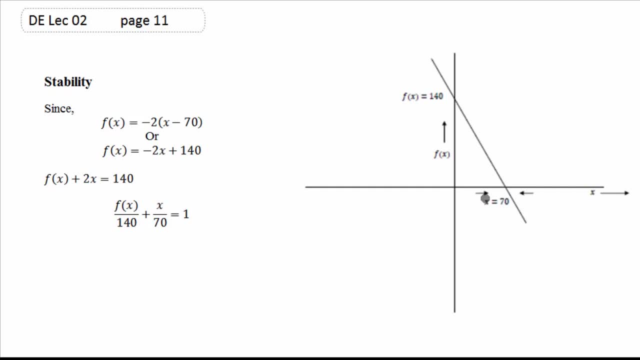 You will apply this arrow from left to right. If the value of your function is negative, below the horizontal axis, then you will apply it from right to left. So whenever these two arrows are coming towards each other, then at the point where they are coming towards each other, 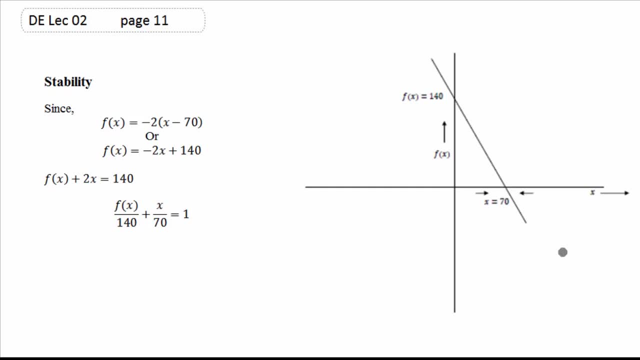 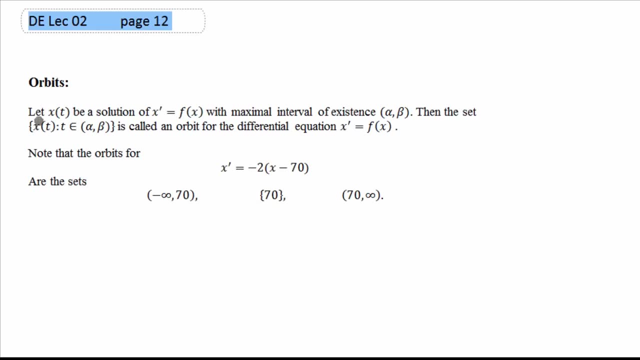 you will say that this is a stable point. Clear, Now let's talk about the orbit. Xt is the solution of any autonomous differential equation with maximal interval of existence- alpha, beta, For example. we just checked Newton's law of coulomb. 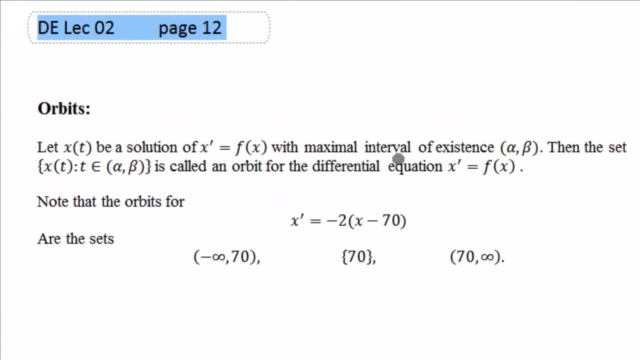 that autonomous differential equation. For that the interval of existence was minus infinity to infinity. Now what we have to do is we have to do that, then the set Xt we have to make the set of this interval of existence. So we have to divide the entire interval into subintervals. 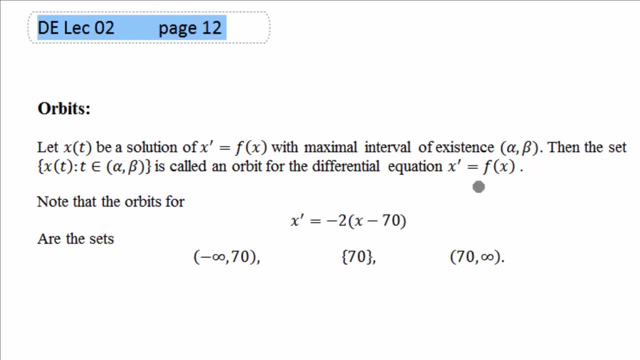 So you can say that all those intervals are the orbits of that differential equation. For example, the orbit for this differential equation is minus infinity to 70.. 70 is not included in it. One is 70,, that is, it is a singleton set. 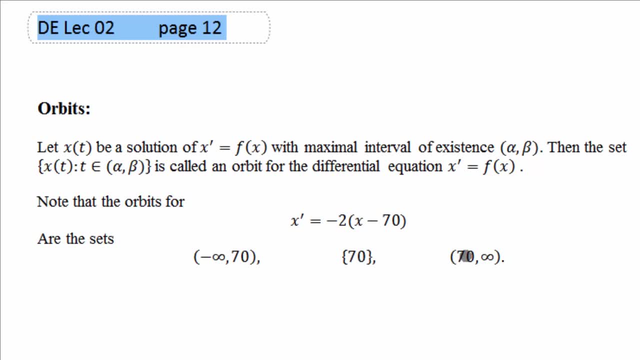 in which there is only one element- 70.. And one is from 70 to infinity. These three are its orbit boundaries, Because for this differential equation there was only one equilibrium point. That is why it has these three boundaries. I hope that you have understood this. 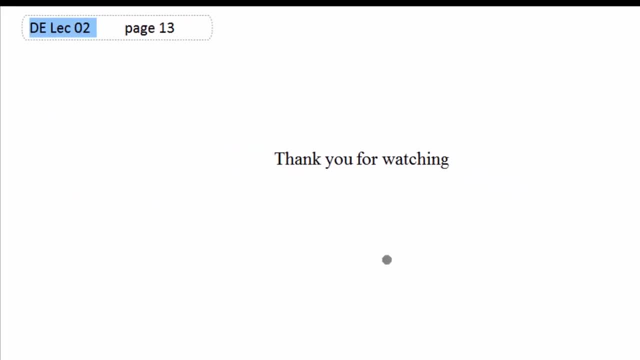 I will be waiting for your feedback. Allah Hafiz. Subtitles by the Amaraorg community. 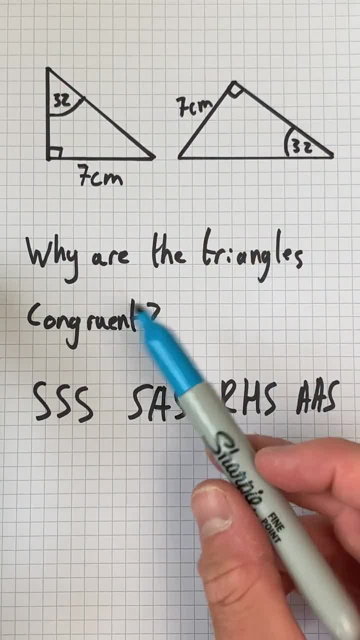 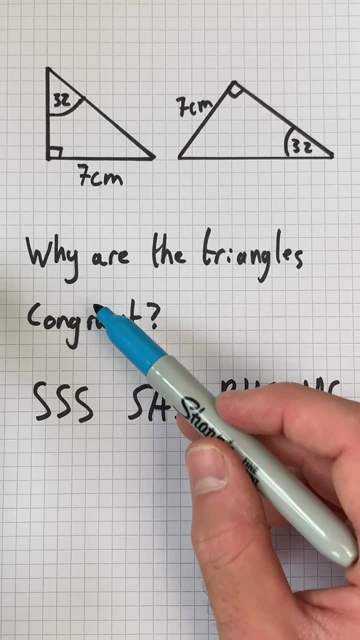 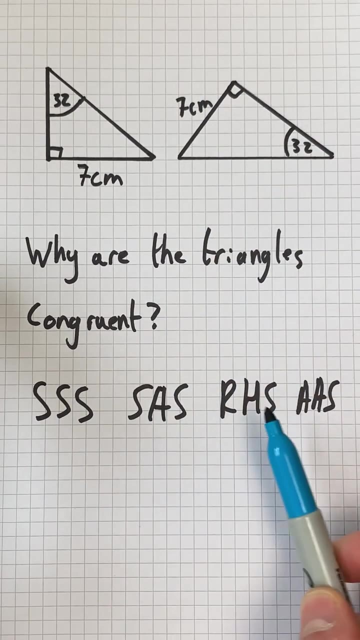 This question gives us two triangles, and then it asks us to explain how we know that these two triangles are congruent. First of all, when two triangles are congruent, this means that all of the sides and all of the angles are identical. They're the exact same triangle. There are four different ways. 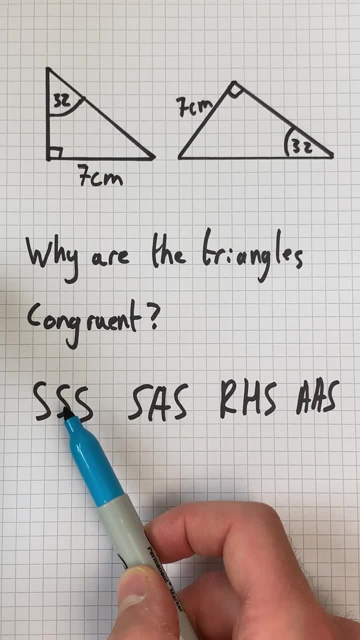 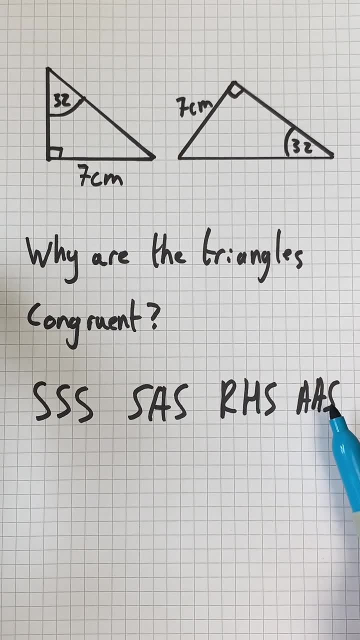 to prove that two triangles are congruent, Proving that they have three sides that are the same: a side, an angle and a side, a right angle, a hypotenuse, and a side, or two angles and one side. So let's see what we know about these. 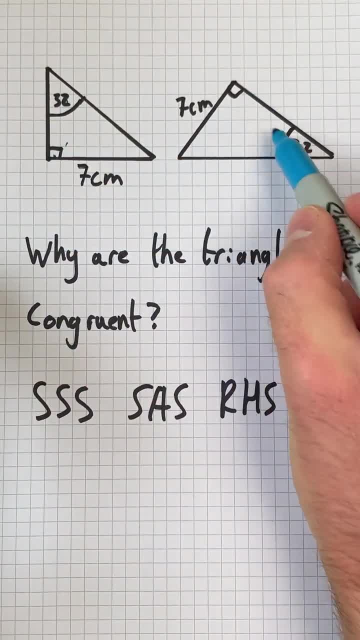 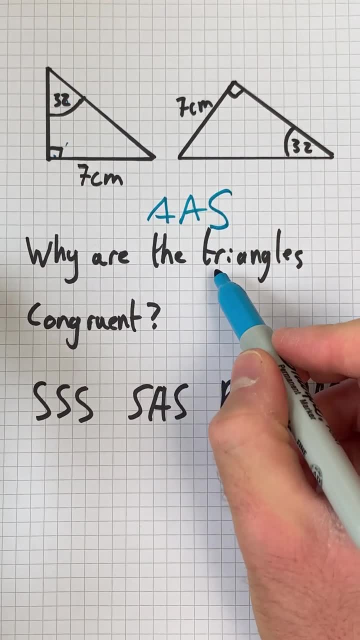 two triangles. We know that they've got two angles that are the same. they both have a right angle and a 32 degree angle, and we can see that they both have a side length being the same as well. As a result, these two triangles are.